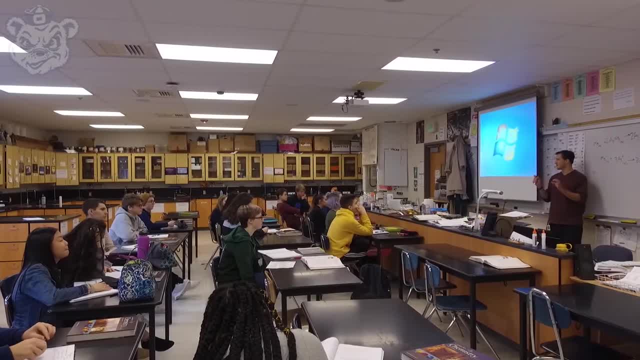 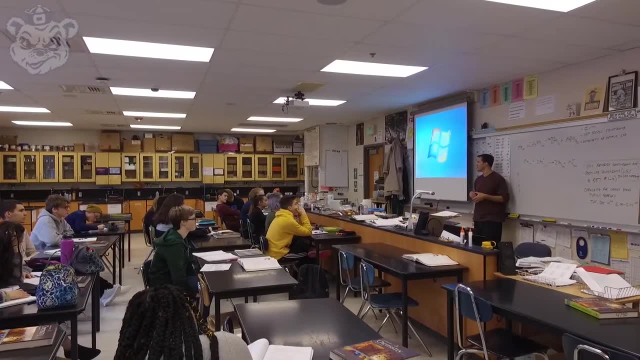 Yes, Well, if there was, if it wasn't part of that chemical reaction, So it could stay solid and so it would react It also. but if it was aqueous it would not be reacting. If it was solid it could be, but possibly not. We need to see what the actual reaction. 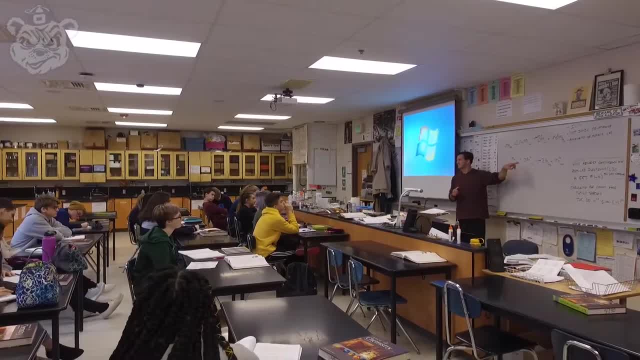 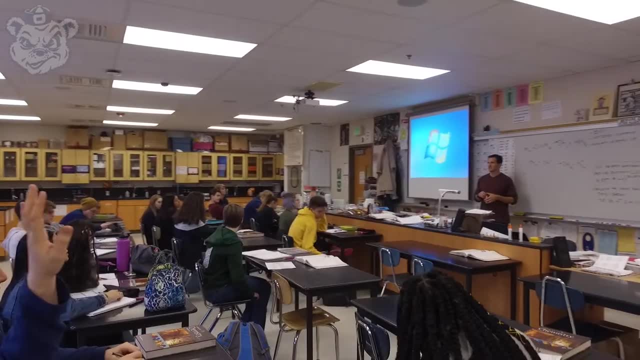 would be. That's what you guys are going to look at right now- is actually what this reaction- I'm not going to use silver, We're going to use six different metals and actually see what that single-split reaction is going to look like. okay, Yeah, right. 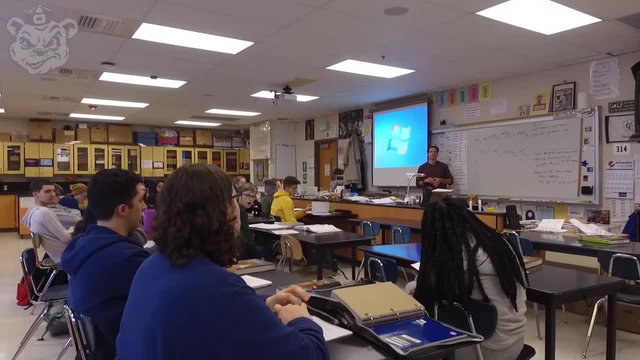 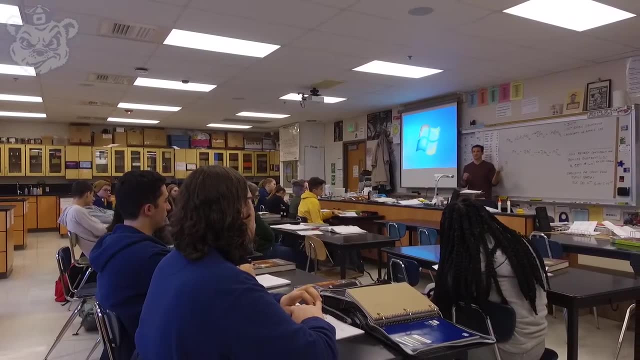 Why are the electrons changing again? Is it because of the pop equation? That is a great question. Any time we see a reaction spontaneously happening, it's because those products are lowering energy or it's more stable. So it's more stable for magnesium. 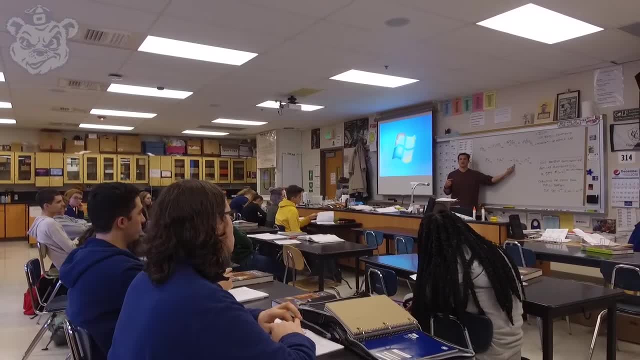 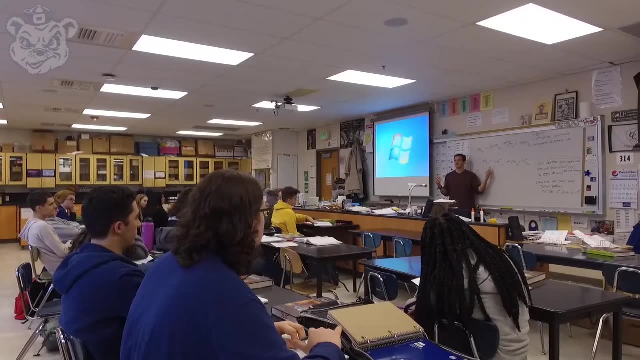 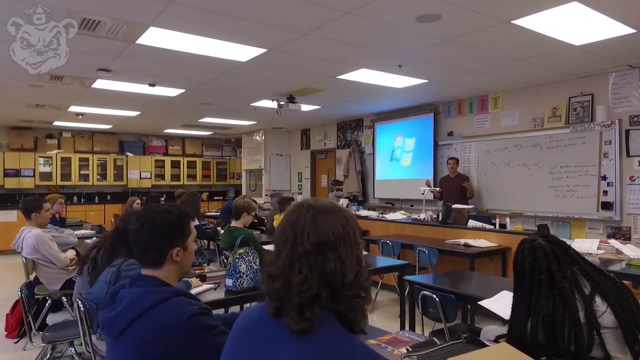 to be oxidized than it is for the- And so all of this relates directly to what we were talking about on Friday- is which of these two metals has been around longer- Silver, Silver- We read about silver in antiquity. It's been around for a long time. It's a precious. 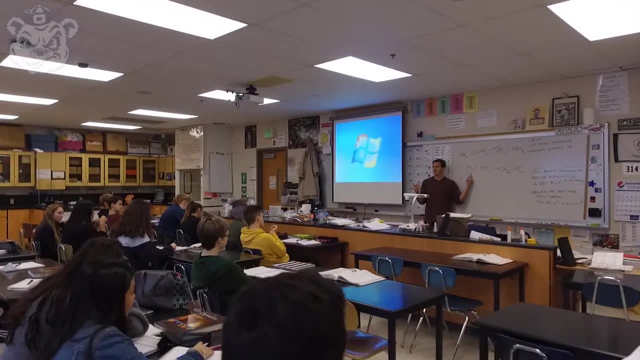 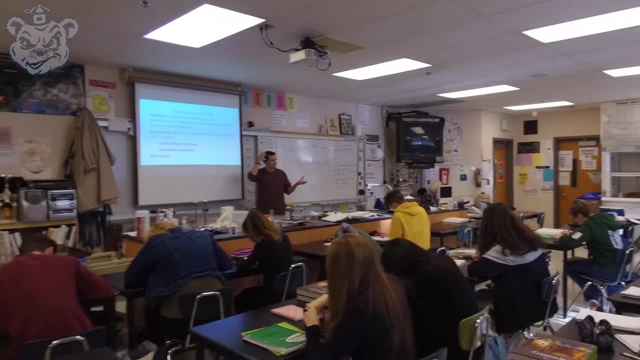 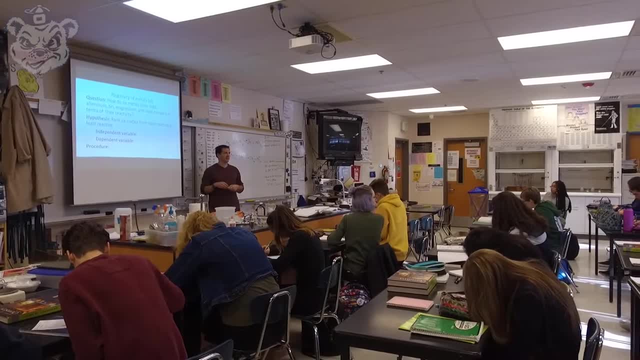 why things are going to react. So our question here is: how do these six metals- when you use zinc, lead, aluminum, tin, magnesium and iron, compare in terms of their reactivity? They're reacting with other salts that are around them. And what I want you to do for a hypothesis here is: don't put it in if-then-because-fold, like you normally would, where you would put it in if-then-because-fold, Because if you put it in if-then-because-fold, it's not going to react. 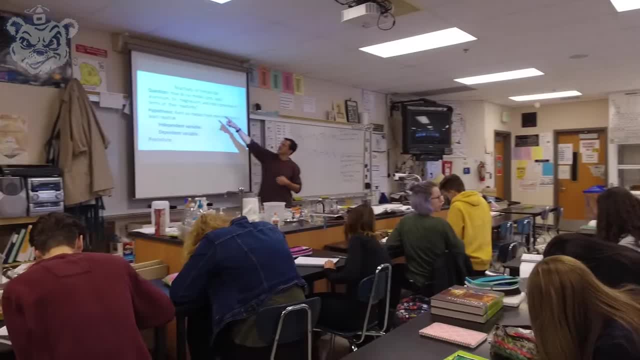 If you put it in if-then-because-fold, it's not going to react. If you put it in if-then-because-fold, it's not going to react When you're saying you're going to depend on a variable and you depend on a variable. 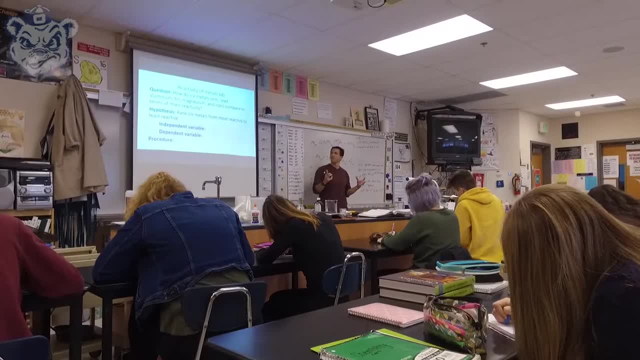 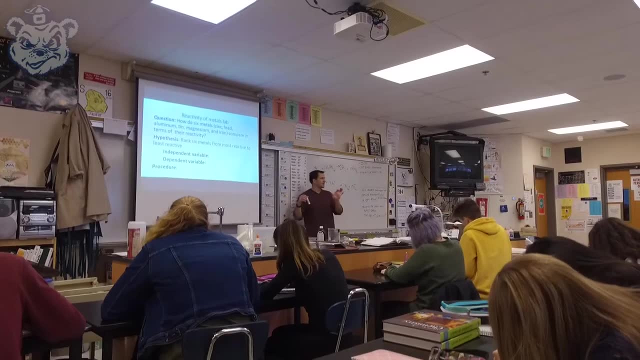 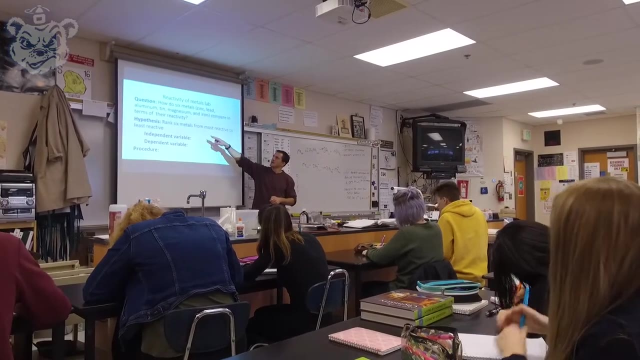 and when you think are going to happen, the relationship between those. I just want you to rank them So based on what we've talked about. we'll talk about it on Friday, So I'm going to go ahead and show you the relationship between the two. 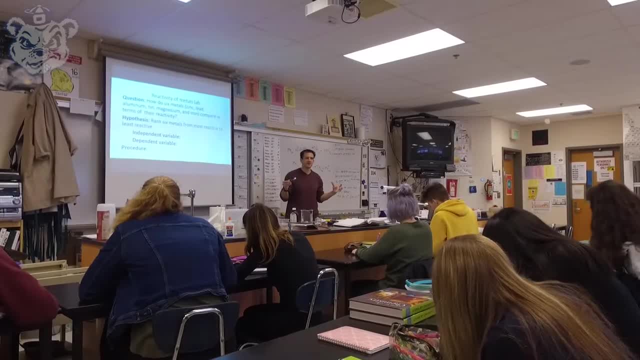 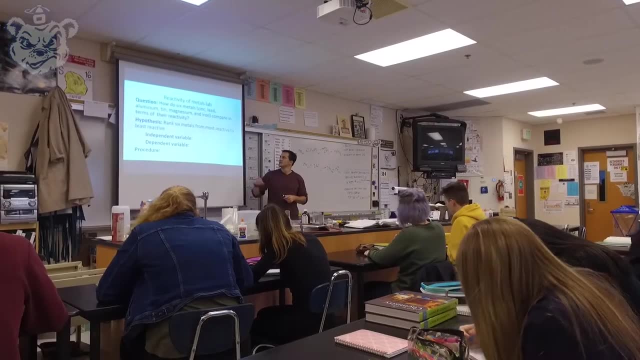 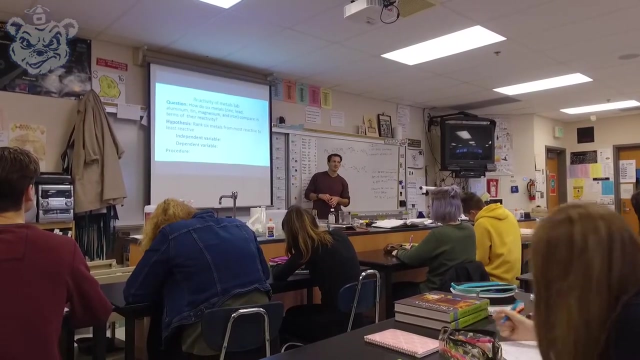 So the relationship between the two, with regard to how long metals have been around, based on your experience with boats, the copper cycle labs and other labs, Once you go from the most reactive to the least reactive metals, And then, after we talk about the procedures and you know what you're doing, 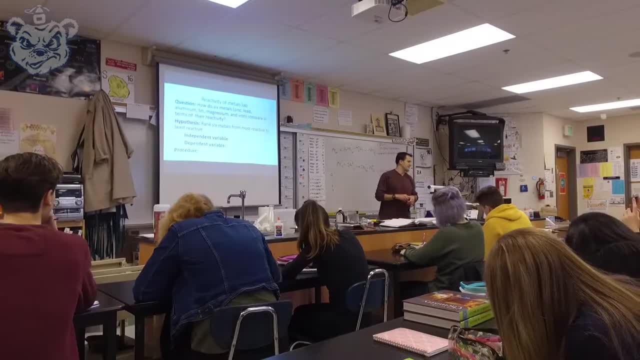 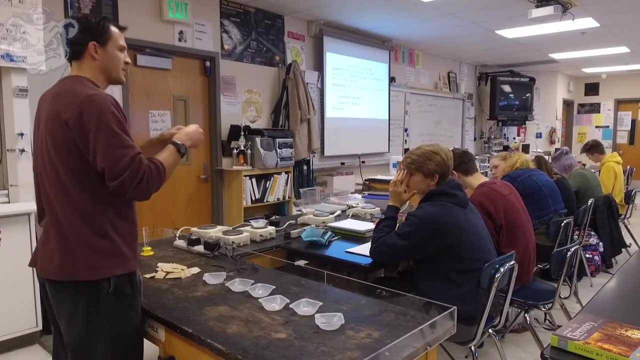 then you can write in what you think is the independent and independent variables. So for each of the metal samples you just need one of these pieces of it, And you want to make sure that there isn't an oxide layer on here, so there's also pieces of sandpaper. 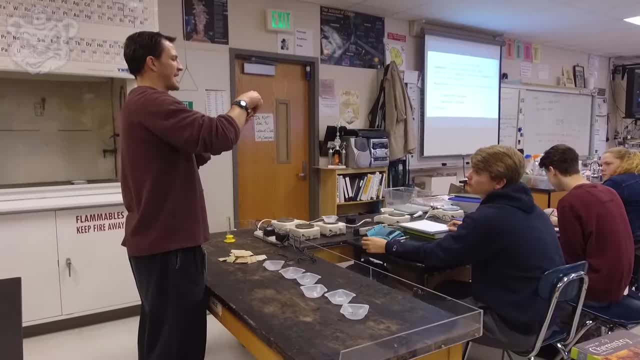 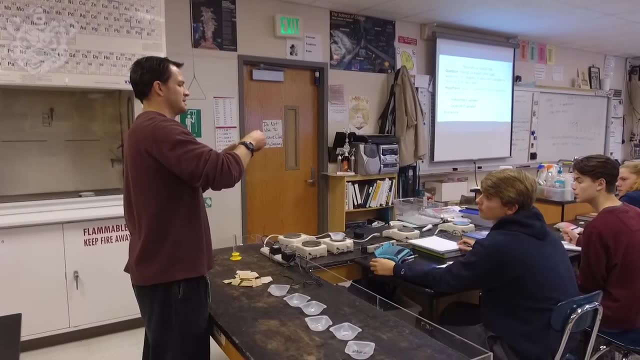 What you can try doing is you can sand the whole thing or, if you want, to try sanding just half of it to see how the oxide layer reacts versus the sanded part of it. So, even if it doesn't look like there's anything on there, you just sand the end of it on each of these. 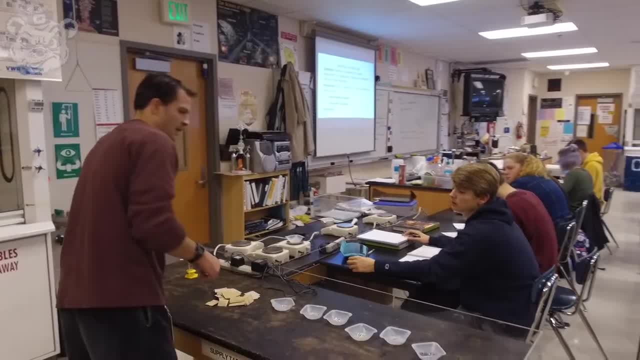 Then you're going to put that into a test tube And what I recommend doing is taking these either two at a time or having each be separated, So that's probably the easiest way to do it. person from your lab group come over so you don't get it confused, because they 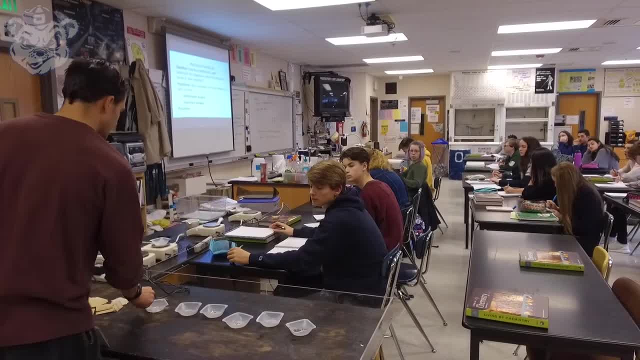 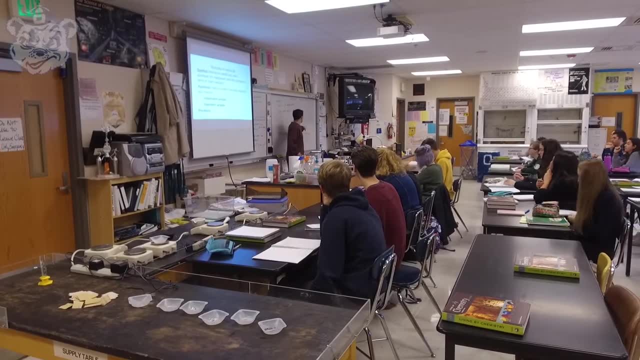 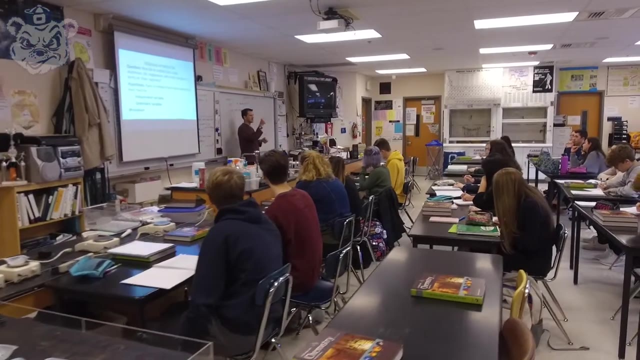 all look fairly silvery, like silvery metals. so you know what they are and then you can arrange them. so you know what is where these up here are arranged, based on atomic numbers. you can do it alphabetically if you want to label on a sheet of paper which one is in which test tube or a masking tape to make sure you know which is which. 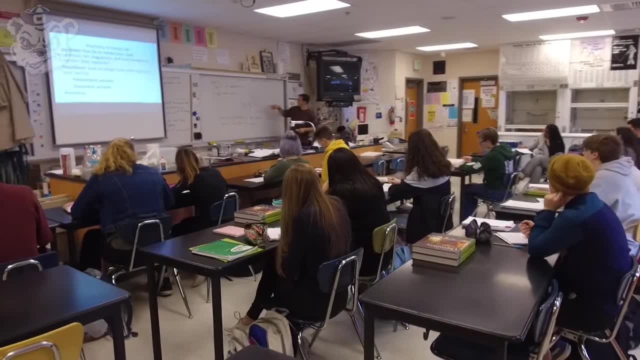 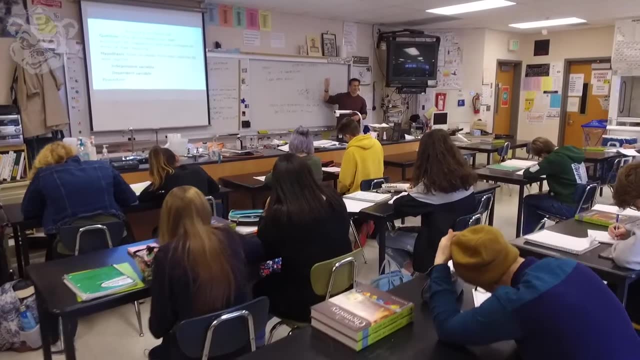 and then you put your metal on the bottom of each of your test tubes and then you put about 45 milliliters of copper sulfate, just cover it up. it's just enough to cover up the metal sample, so you shouldn't see it reacting. and then 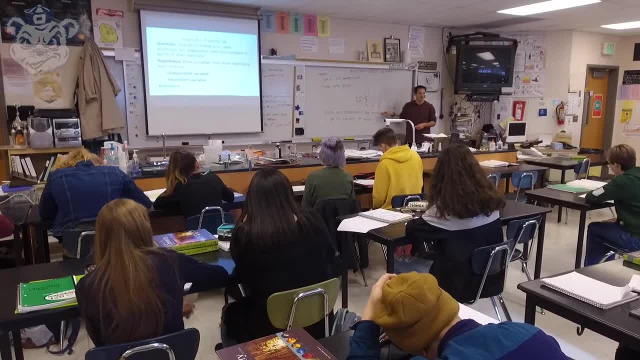 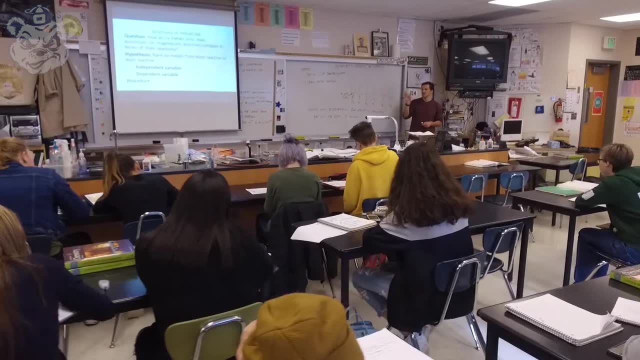 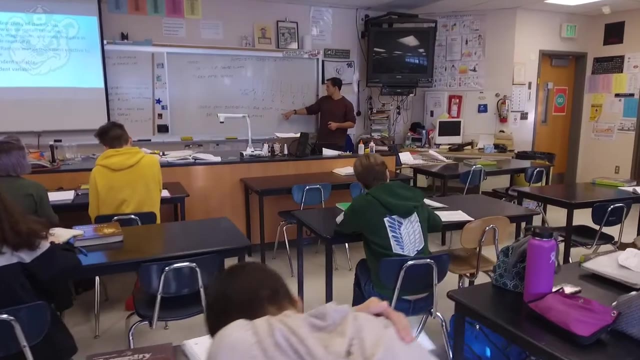 for each of those. as you put the copper sulfate in, observe it for a minute or two on its own and how fast it starts reacting. what you see happening? you see bubbles coming up, you see color change, you can feel the temperature change. so it's some evidence of a chemical change. and then, after you let that, 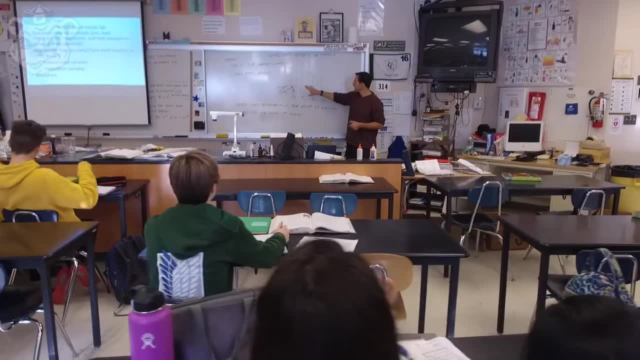 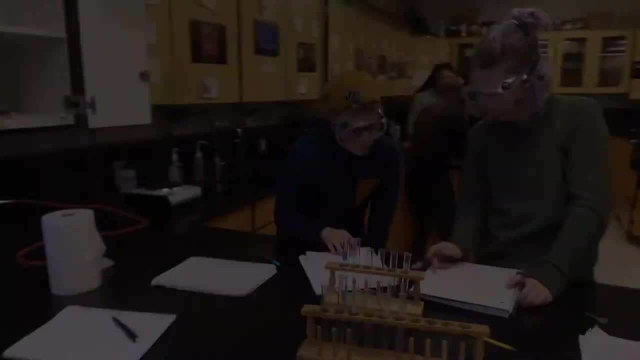 react for about one or two minutes, then you can move on to the next one and then, after you've got them all there, after that about you know 10-15 minutes, and kind of make your observations about all of it. actually I said aluminum in there. 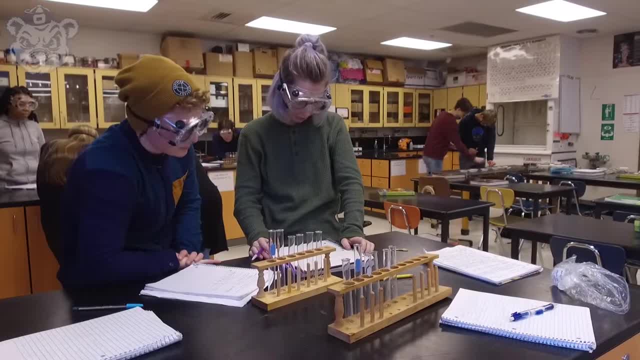 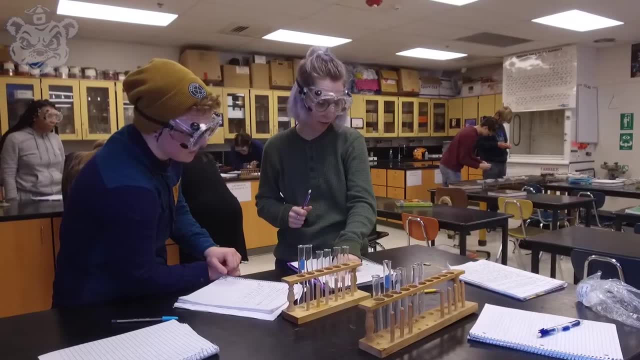 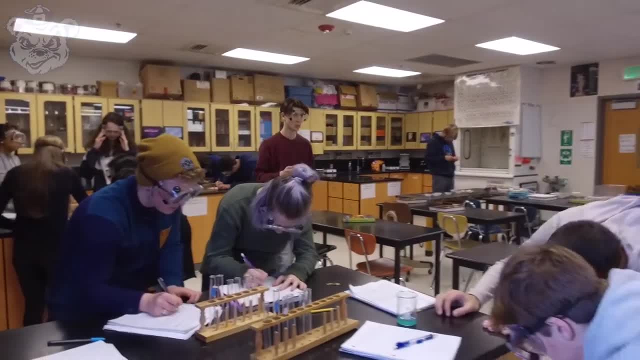 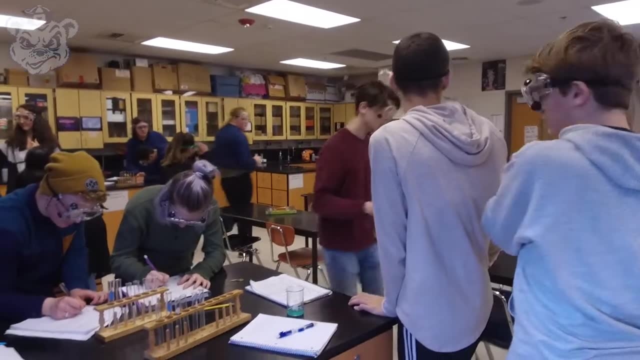 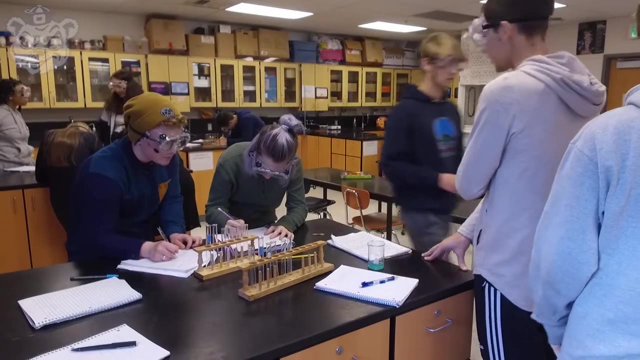 got it. okay, all right, we just want don't have a lot, all right, so 25 milliliters. oh my gosh, I got ya 25 milliliters. oh yeah, we got 10. should we put it in a tin? yeah, it's 25 milliliters. 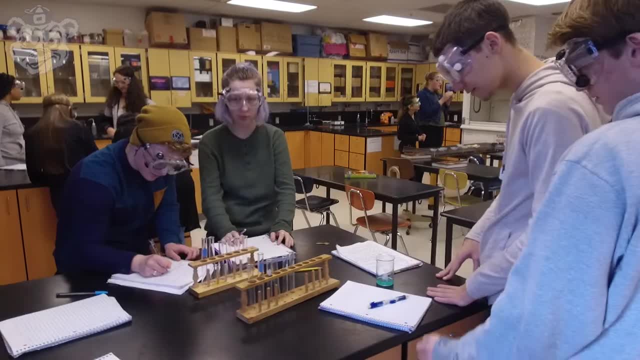 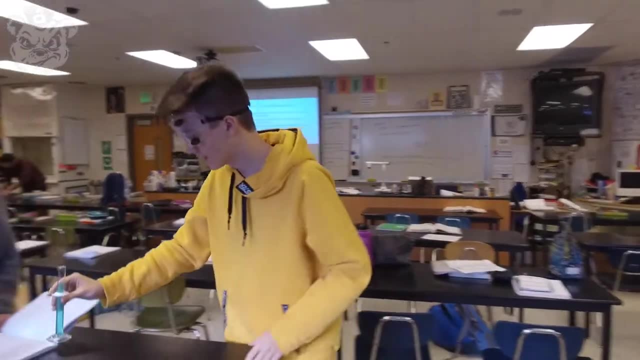 so yeah, and then we divide it up. alright, we'll keep it there, okay: M-G-A-L-F-E-S-F-E-N-E-G-A-S-E-N-E-F. so should we go with the name? definitely, we need four to five milliliters in each, so we can do this one first. so this is. 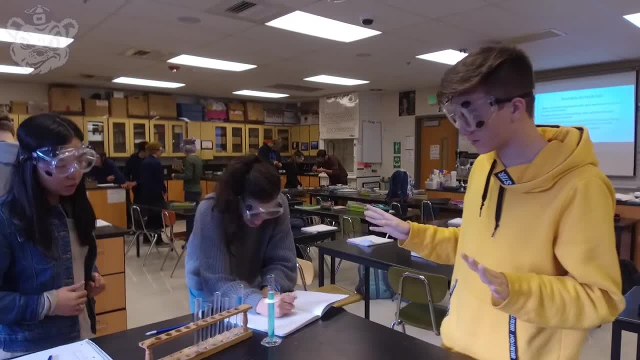 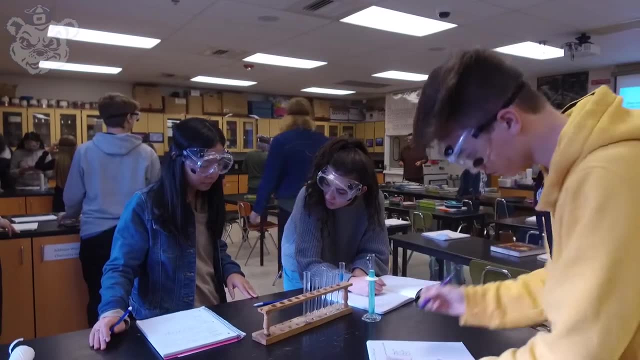 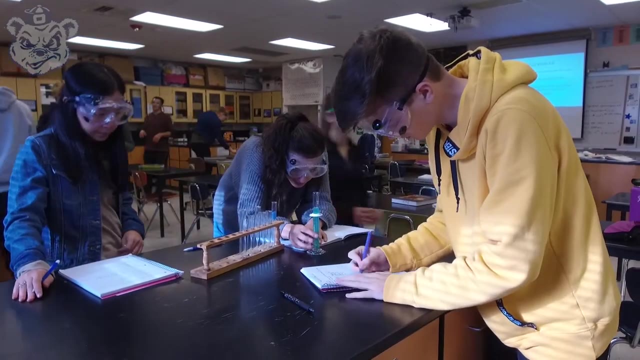 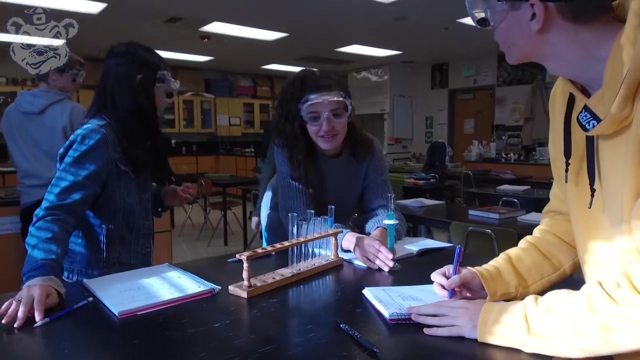 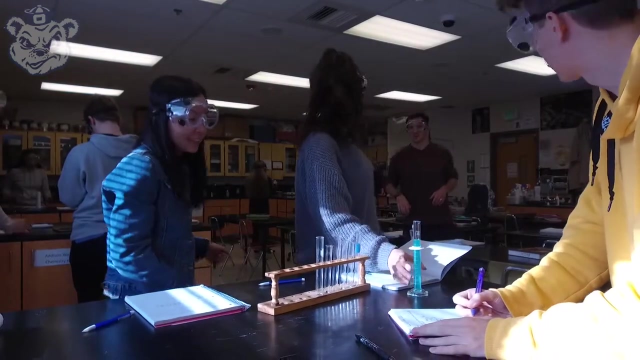 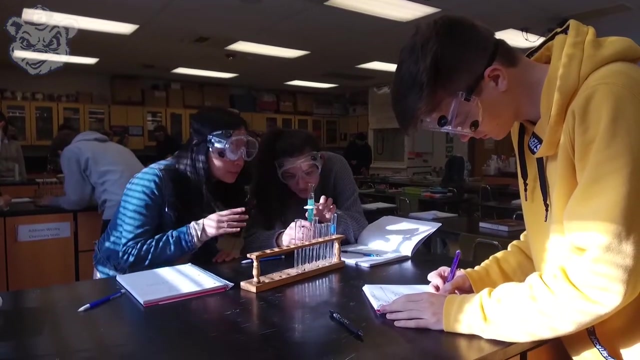 what we got to be like. careful though that, yeah, that's a lot of pressure. all right, let's do like. tell me for each. i know, but what is this? what do you think this is? so it's about 45, just so it covers up your sample. oh, just so it covered. 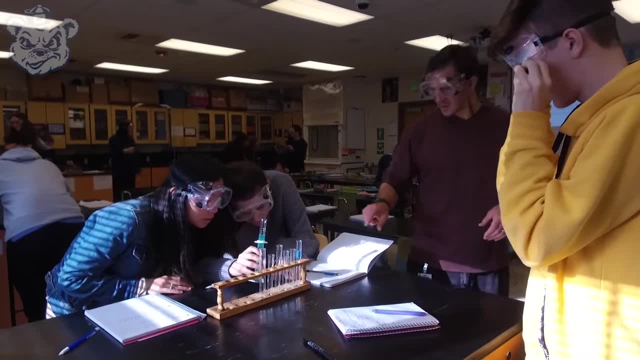 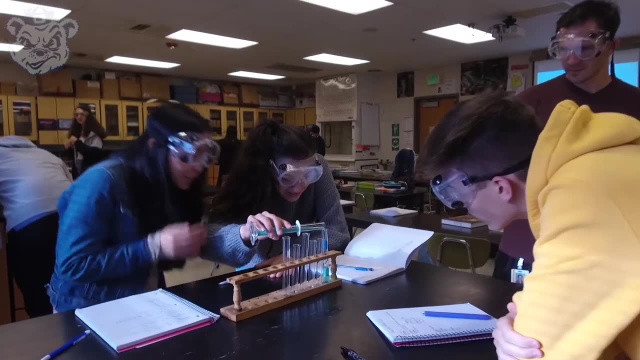 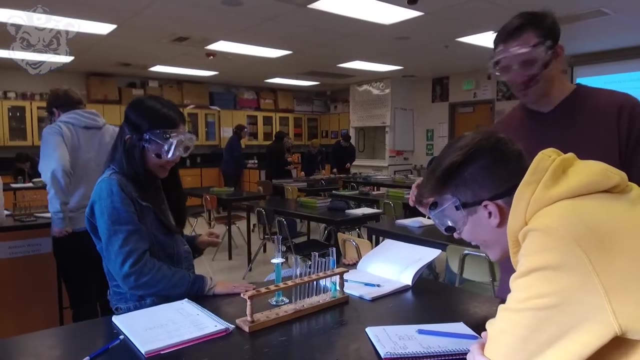 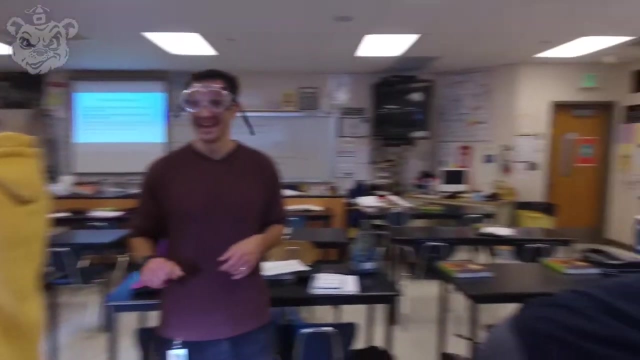 oh, okay, wait, covers it fully. uh, yeah, all right, yep, so we can just pour it in one at a time. yeah, okay, so we're starting. i don't smell, i need to, i need to, i need to, oh, oh, oh, no, that's so much. which one is this one? 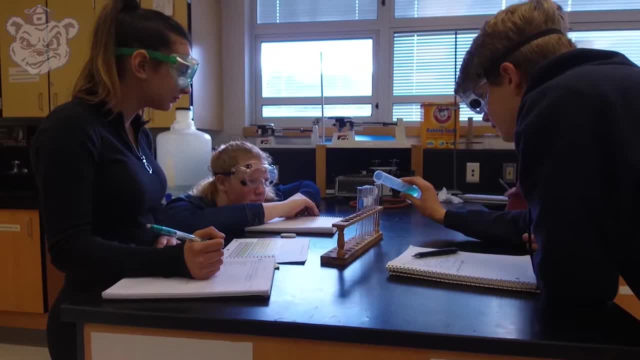 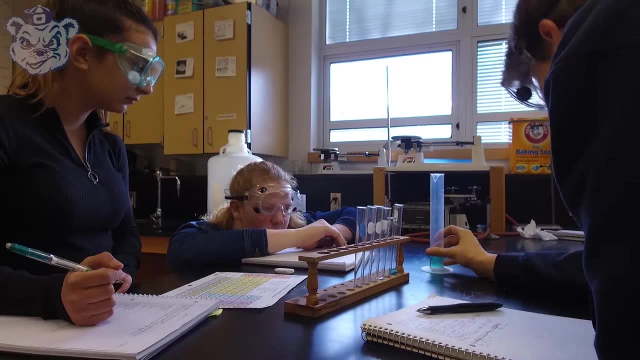 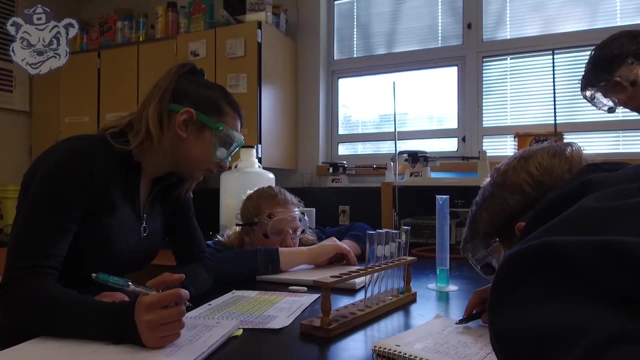 okay, okay, okay, okay, someone else do it. can we just redo it? yeah, you can just redo it. let's just do it i'll. i'll get another one. what are you doing? oh wait, something's really hard. i already have terrible. that was funny, that was so bad. 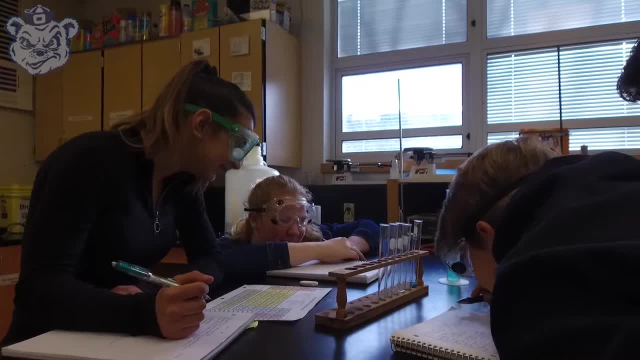 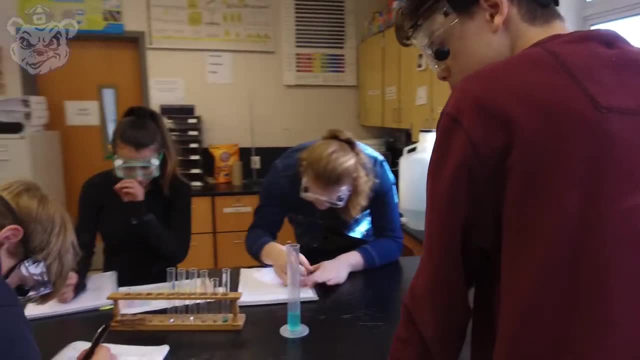 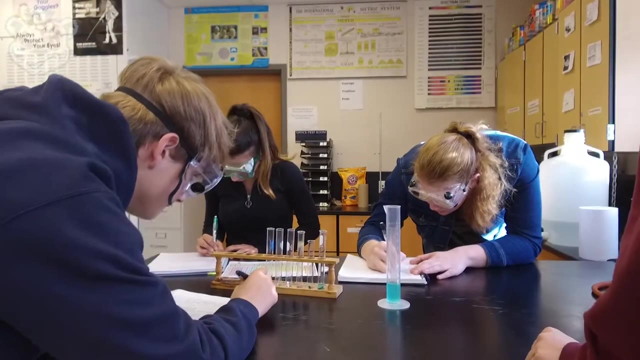 i love him. i haven't dealt with him in a long time. got it, got it, mom. what did you say? nothing that she's gonna like stop pouring and she'll. yeah, she kept pouring it. i'm not gonna lie. it's definitely looking good. okay, all right, all right. 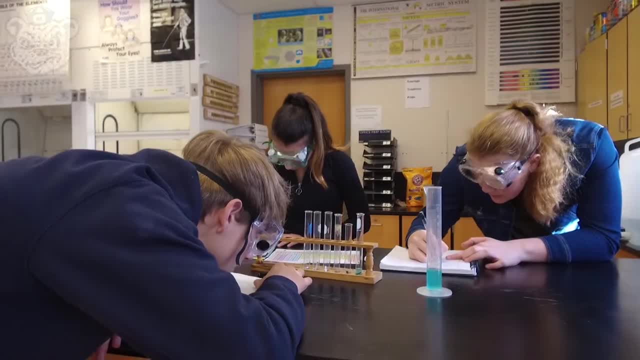 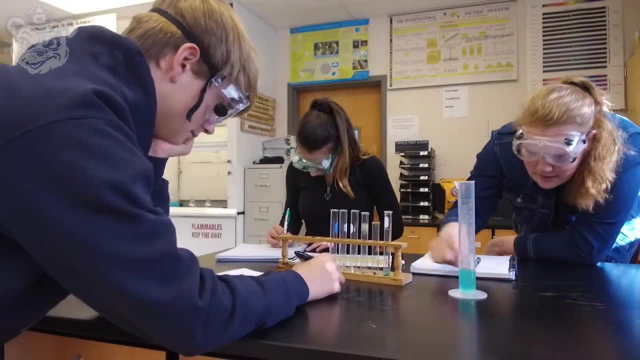 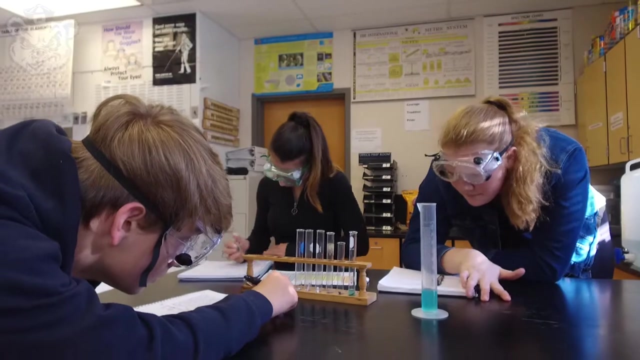 what we're supposed to do for like one minute. can we try? just you did it. maybe it's getting a little lighter. it looks like it's at a certain 19. stop. okay, maybe it's actually the same color. stop see, it's harder than it looks. 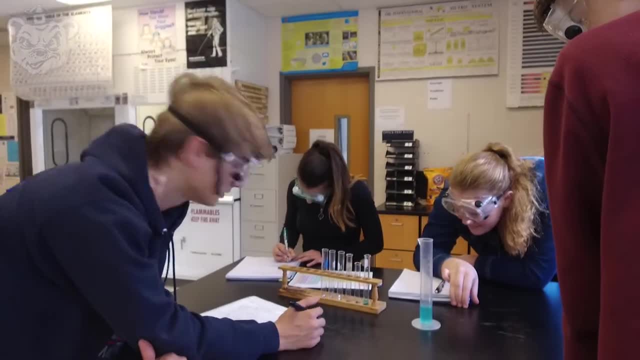 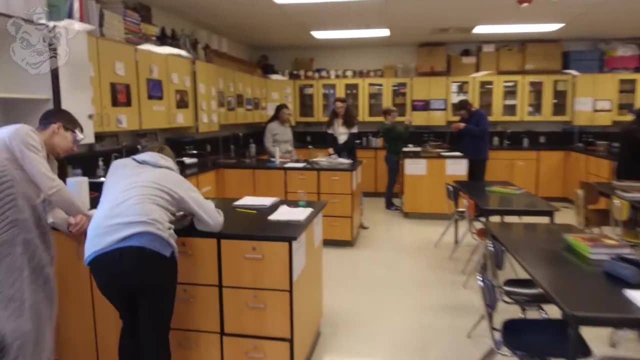 oh, no, that's so hard. you did the same thing. no, it's okay. it's okay. you know what it's, whatever it was at the bottom. all right, amanda, you do this one. show us that you can do it. yeah, do the next. so what is it? 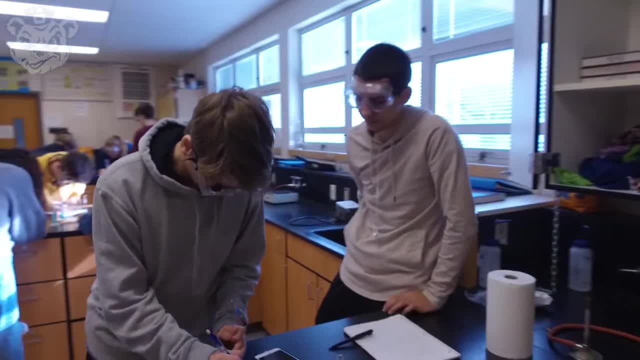 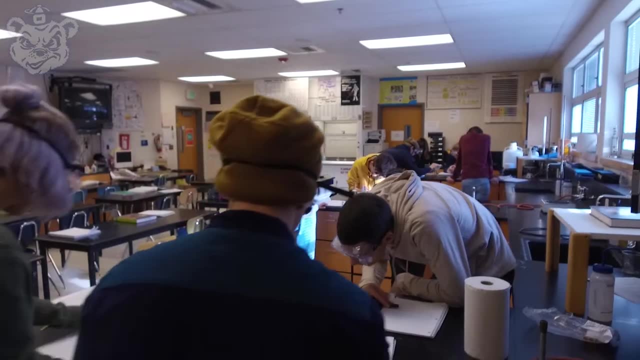 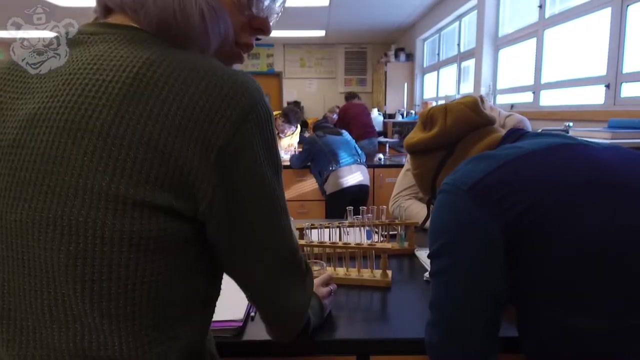 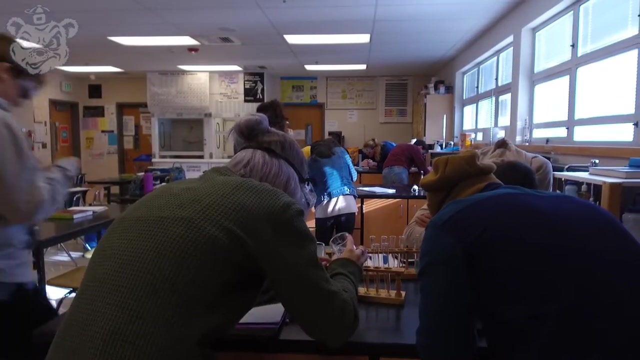 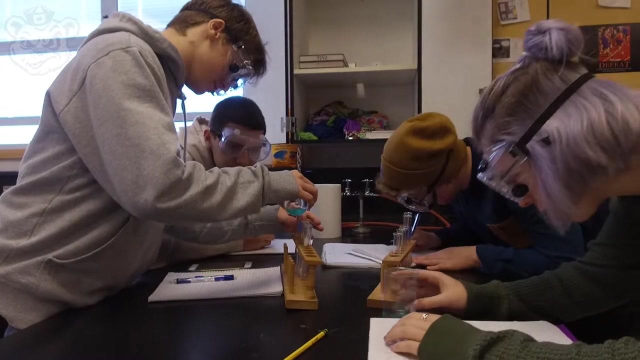 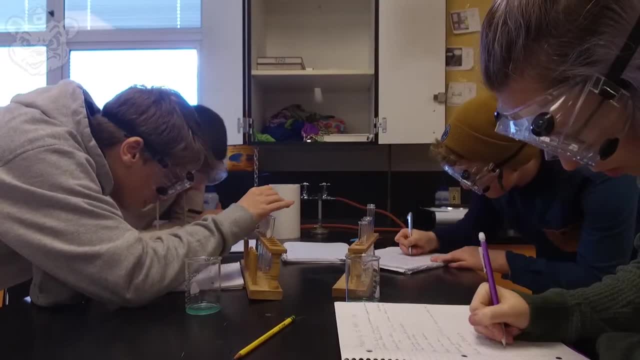 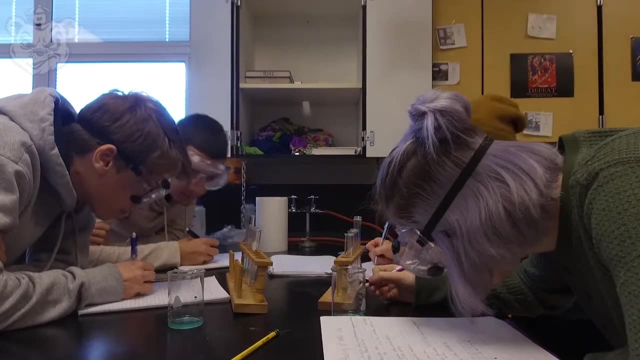 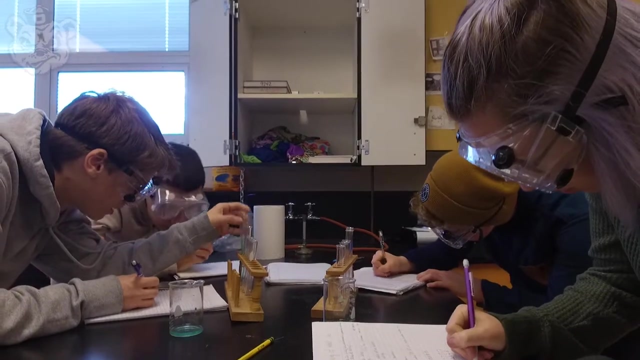 i don't even see it. it doesn't float, definitely, no, no, float. uh, yeah, so it looks like it's turning darker around the edges. no, tiny bit. oh, this thing is turned black. yeah, i got that kind of black. well, it's like the stuff falling on. oh. 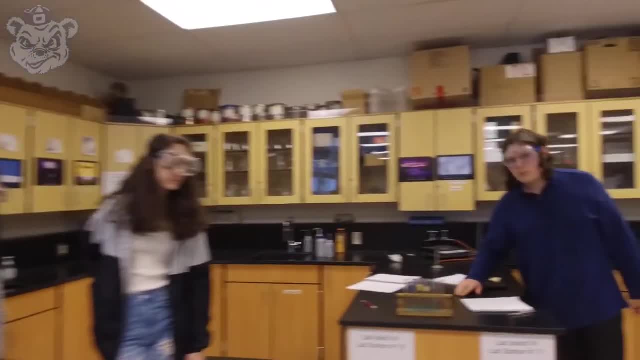 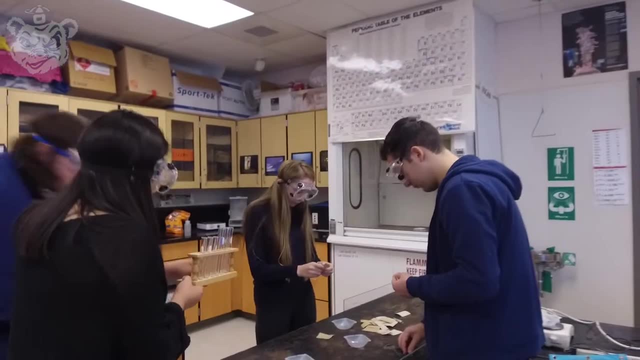 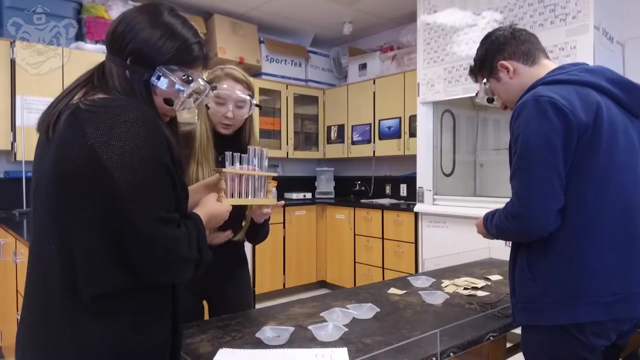 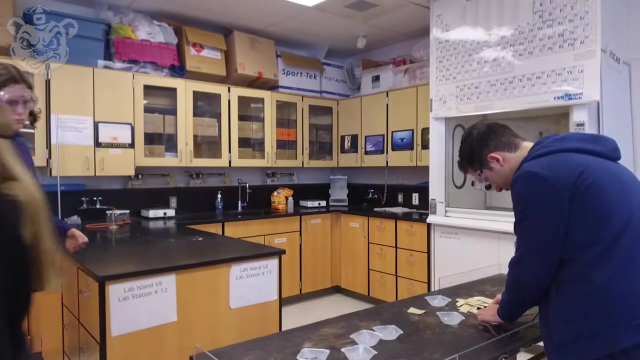 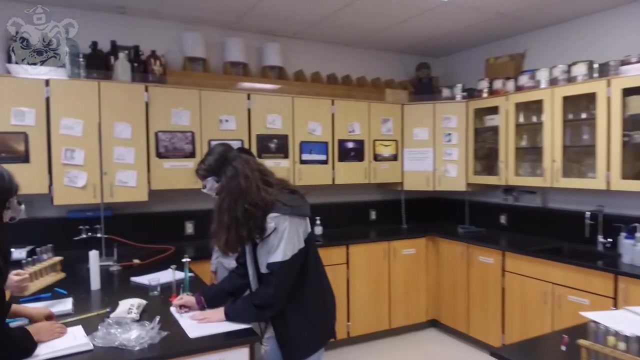 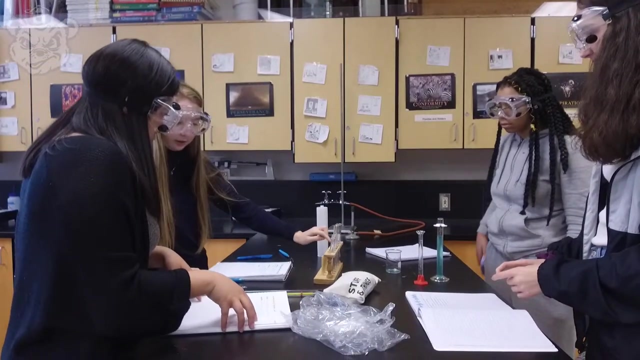 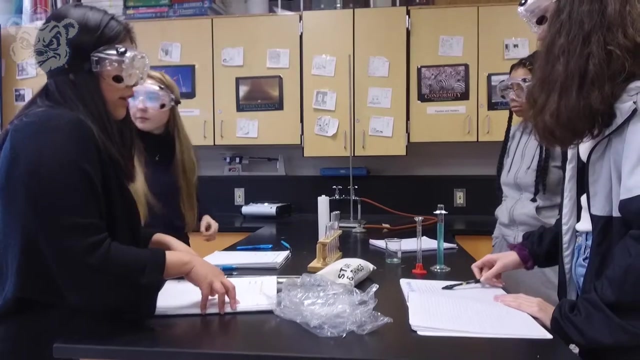 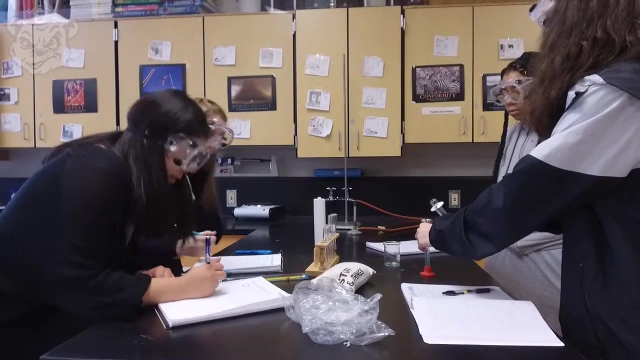 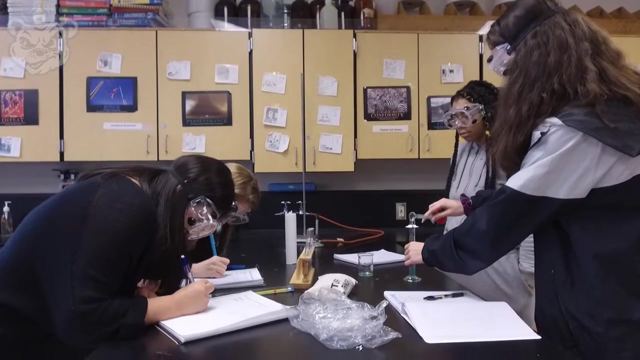 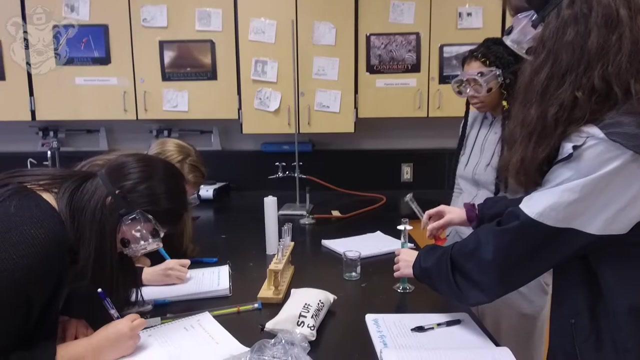 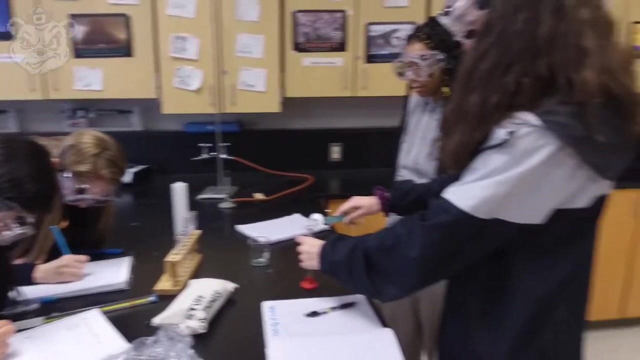 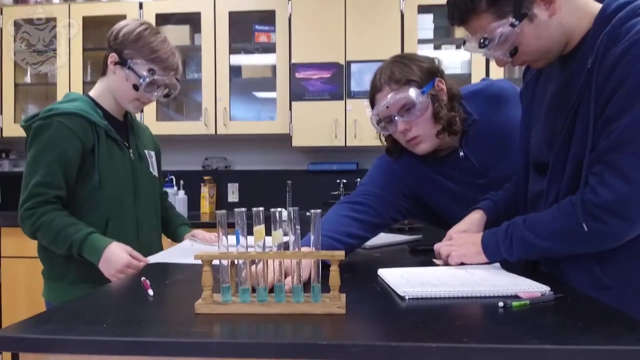 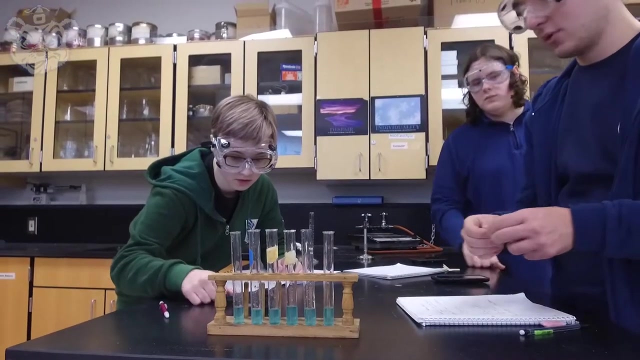 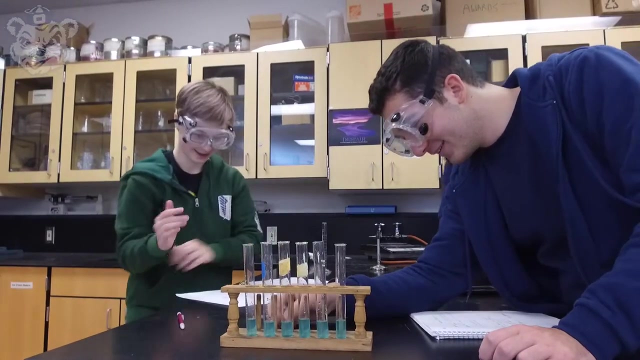 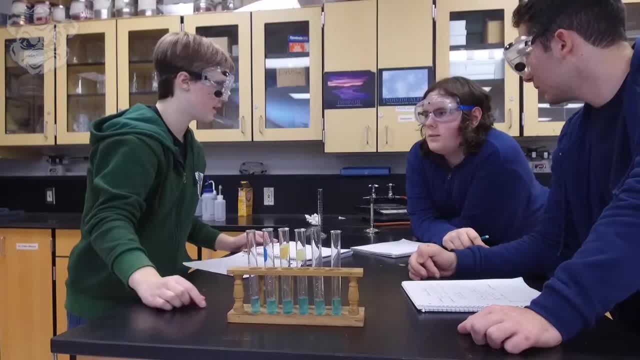 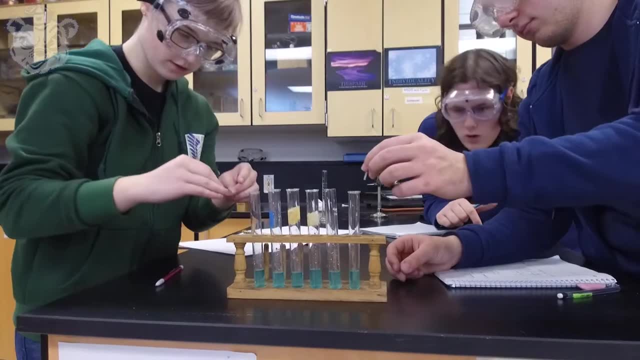 Do we have to drop it in at the same time? Yes, We have to drop it in at the same time. Yeah, they all have to drop it in at the same time. Alright, let me get the timer ready. Yo, what are you doing? 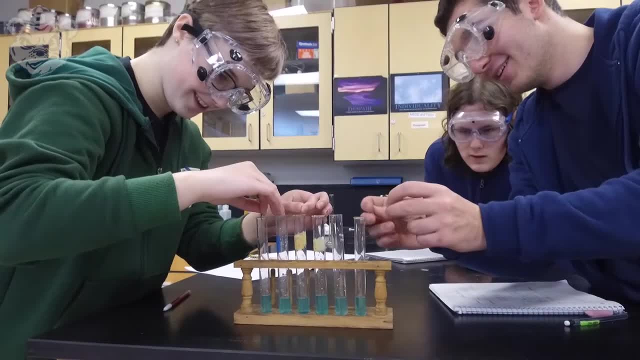 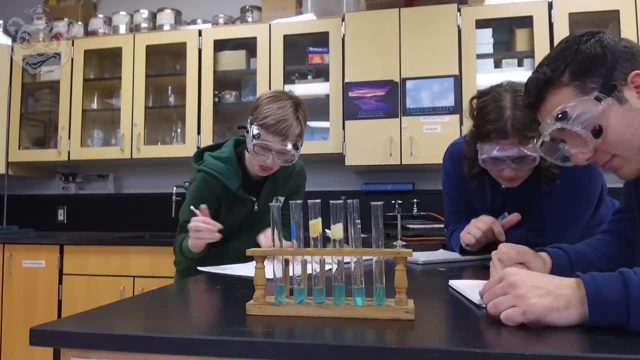 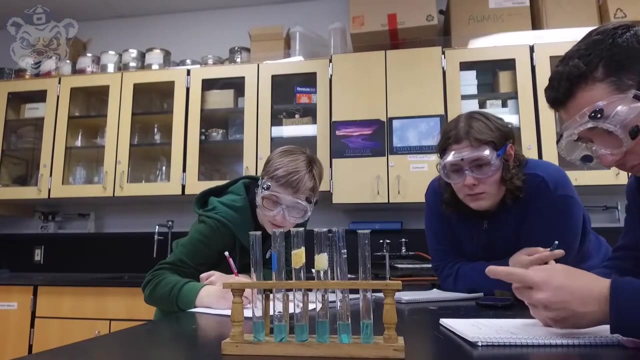 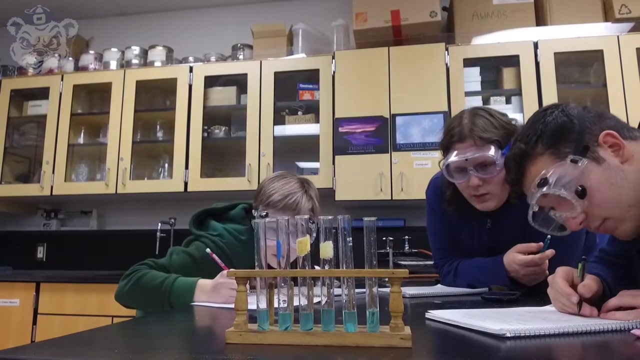 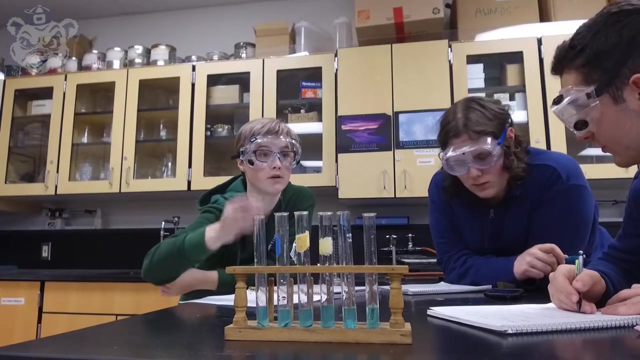 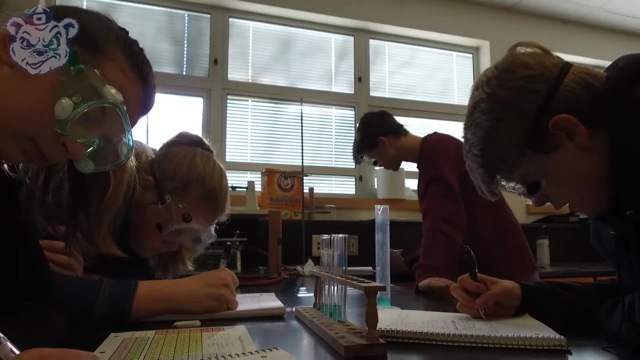 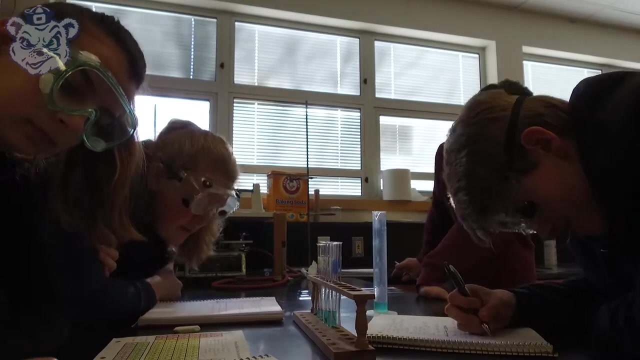 Yes, We don't record immediately. We'll wait for a few minutes. We have it. Yeah, we record for the first two minutes. I'll go On the edges, on the very ends. Okay, Is it turning the color? 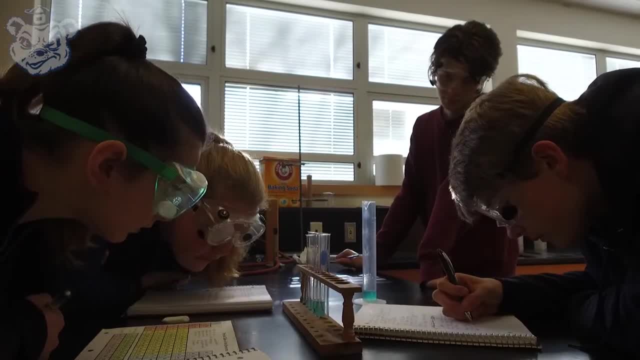 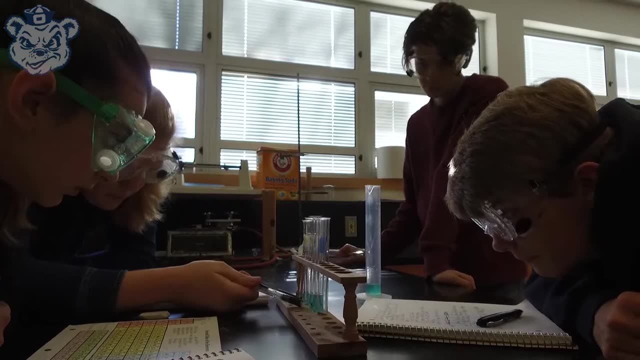 I can't really see. Can you tell what color it is? Oh, it's dissolving. It's more black than that one. They're all pretty much the same color, so it's more black than that one. Okay, One, two, three, four.